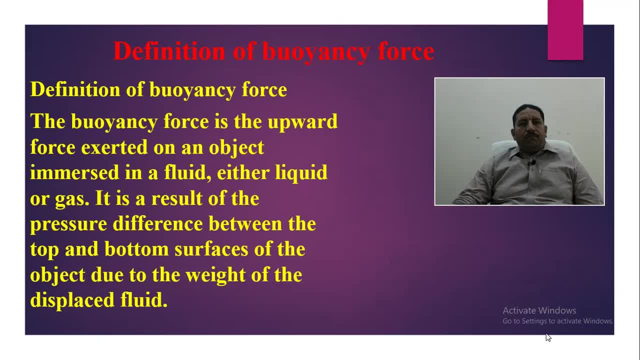 In the name of Allah, the Most Gracious, the Most Merciful Peace be upon you. dear students, Today we discuss buoyancy and key characteristics of buoyancy force. The definition of buoyancy force is upward force exerted on an object immersed in a fluid, either liquid or gas. 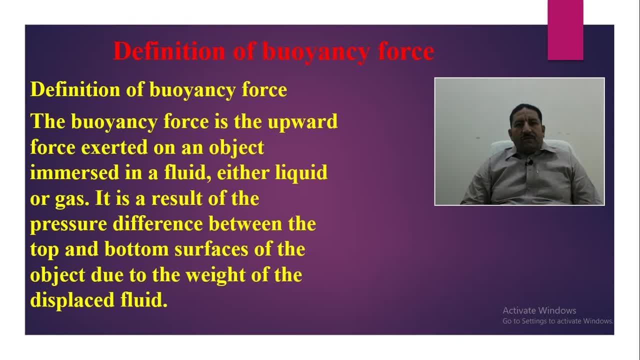 It is the result of the pressure differences between the top and bottom surface of the object due to the weight of displaced fluid. Du�나 Clarifying the pressure from the bottom to the top, that is, the pressure between the bottom and the top. 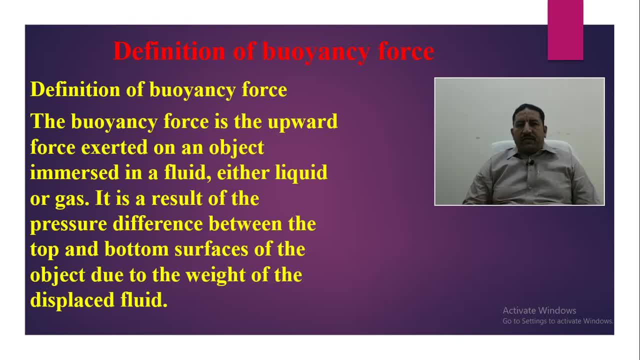 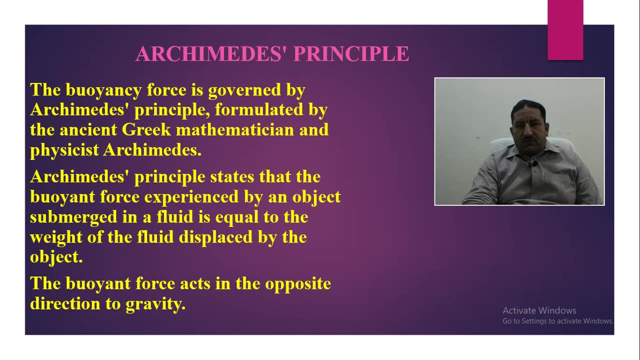 whatever you put in the water, the displaced fluid that is. when you put something in the water, the more the thing goes into the water, the more the fluid moves from the bottom to the side. So this is the reason for the Bionci force. 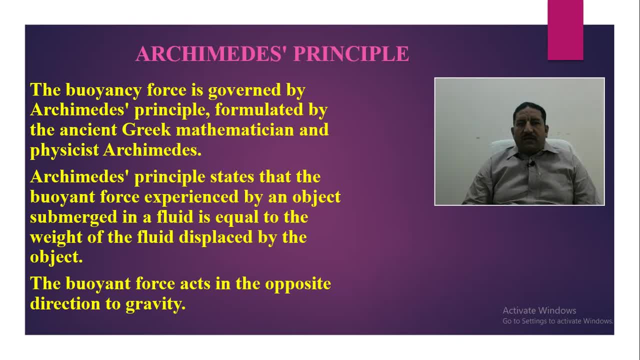 And one of the biggest Archimedes principles is related to Bionci. The Bionci force is governed by the Archimedes principle, formulated by the ancient Greeks, mathematicians and physicists. Archimedes was a great mathematician and physicist. 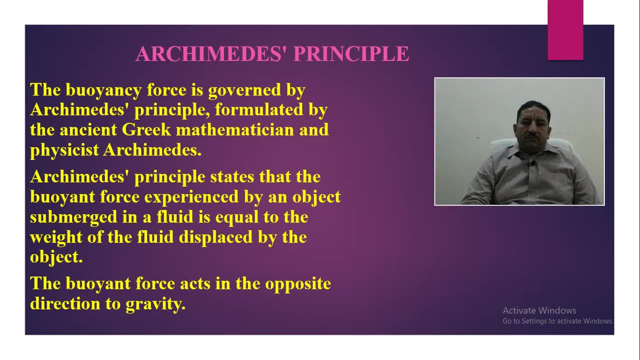 So he introduced an Archimedes principle. According to him, the Archimedes principle states that the Bionci force experienced by an object submerged in fluid is equal to the weight of the fluid displaced by the object. According to him, the force of the Bionci force is the Bionci force. 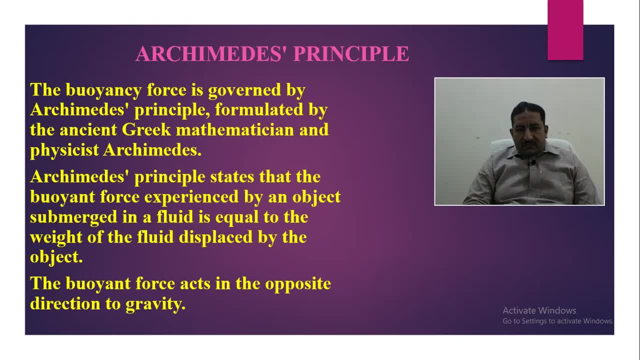 So the Bionci force is the force of the Bionci force, And this shape also connotes that heถ, The Bionci force, is equal to the mass-weight of his displaced object, either it's in water, gas or liquid. 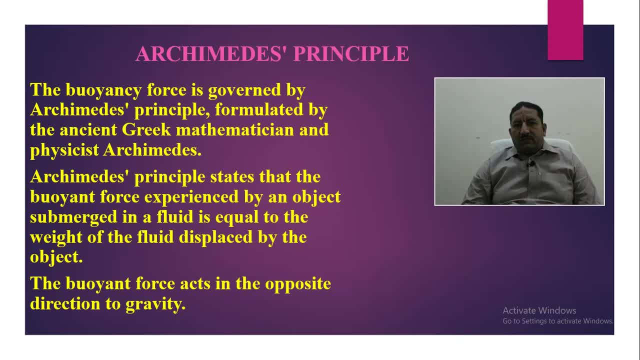 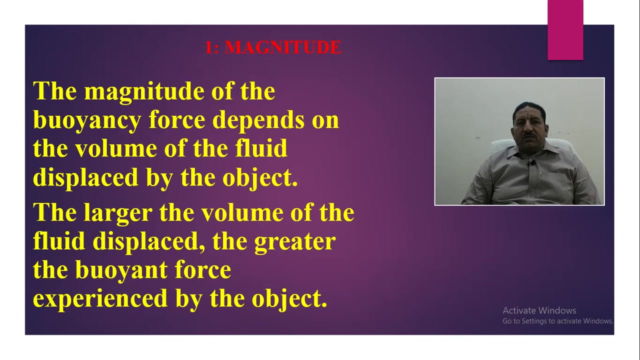 The Bionci force acts in an opposite direction from the gravity. Bionci always acts in the opposite direction from the gravity. The Bionci force is the upward force. The magnitude of the buoyant force depends upon the volume of the fluid displaced by. 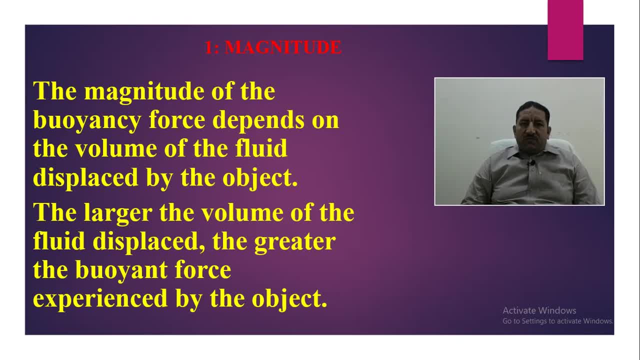 the object. The magnitude depends on the volume of the fluid displaced by the object. The larger the volume of the fluid displaced, the greater the buoyant force experienced by the object. The greater the volume of the fluid displaced by the object, the greater the buoyant force. 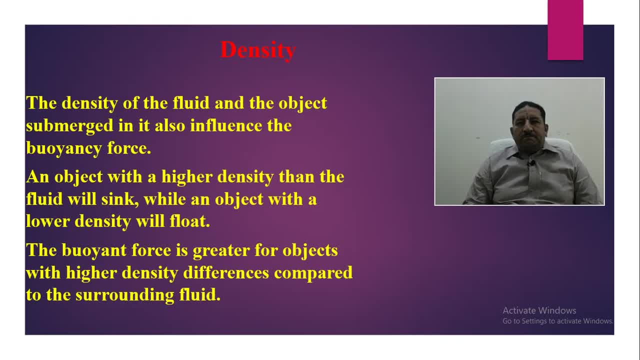 experienced by the object, The density of the fluid and the object submerged in the water. It also influences the buoyant force. An object with a higher density than the fluid will sink, while an object with a lower density will float. It means that another action has been done in this, that is, the density of the fluid. 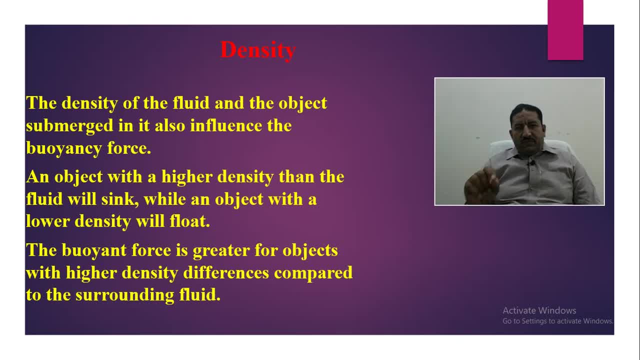 and the object, The density of the fluid and the object that you will put in the object or the fluid, the density will also be affected. Theố ï balance of the sound and the sound is the sum, 1.2.2.4.. 3.4.4.5.5.6.6.7.7.7.6.9.7.8.7.9.10.10.10.11.11.12.13.13.12.14.14.13.14.15. Britt, Commonwealth. 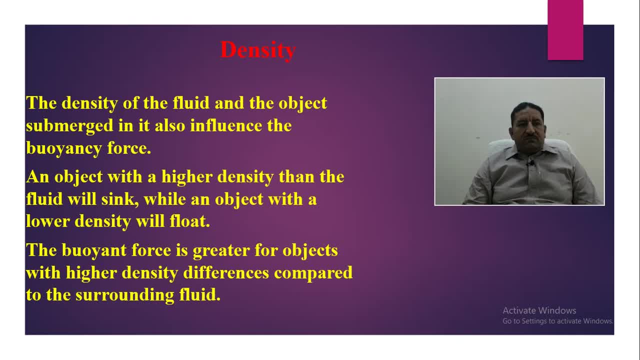 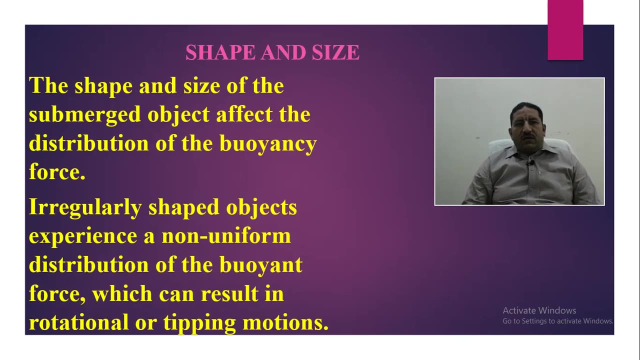 This is because of the density of the object. The buoyant force is greater for objects with a higher density. Difference is compared to the surrounding fluids. Shape and Size. The shape and size of the submerged object affect the distribution of the buoyant force. 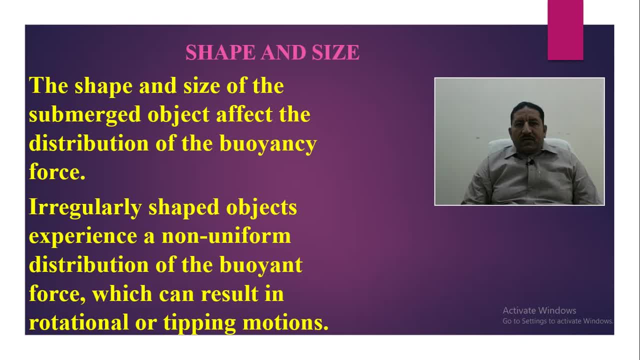 The buoyant force also affects the shape and size of objects. How is it? Irregular shapes of objects experience a non-uniform distribution of the buoyant force, which can result in rotational and tipping motion. Do you know that when a submarine or a submarine has to navigate in the water, 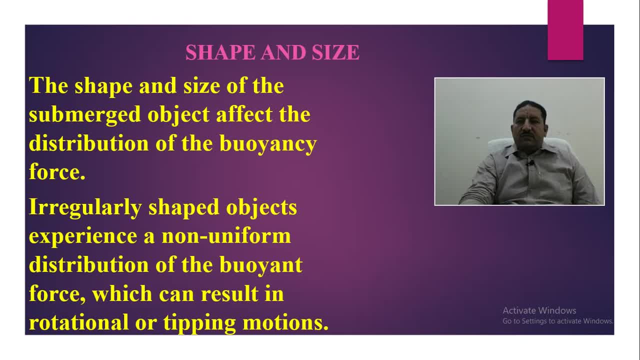 when these things are made, there is a special shape on the surface of the surface, due to which they get as much buoyancy force as possible and help them float. So this is the shape and size of the buoyant force. You can see that there is a needle and it has the same weight. 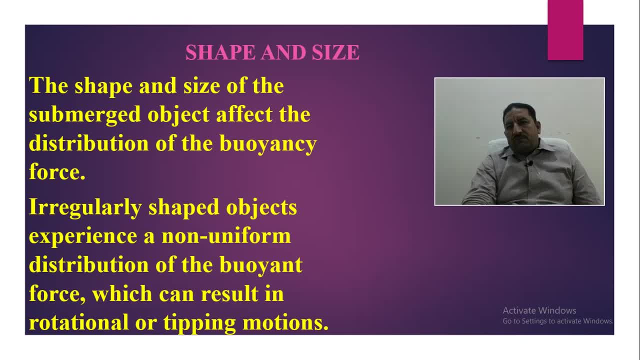 Or you throw the weight of 2 kg And the other one whose volume is more. that is, you throw the weight of a plate, then it floats, But when the water is filled in it then due to its high weight, it will sink. 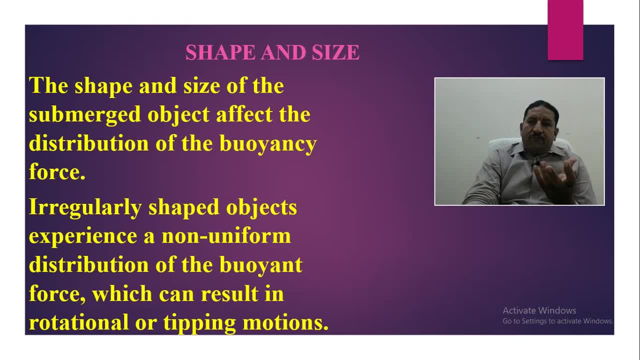 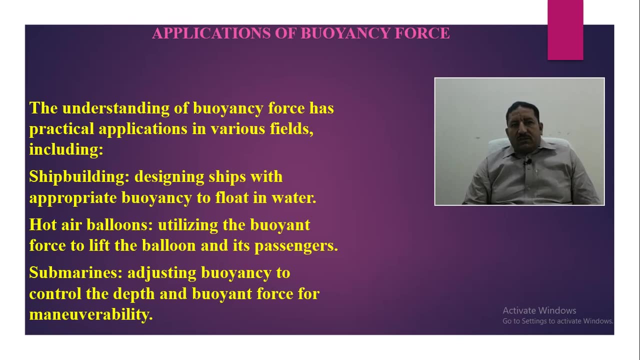 That is, you can say take a bucket and take a weight equal to that which is solid, So then there is a lot of that shape and size. There is an impact in this. The applications of buoyancy force. The understanding of buoyancy force has practical application in various fields. 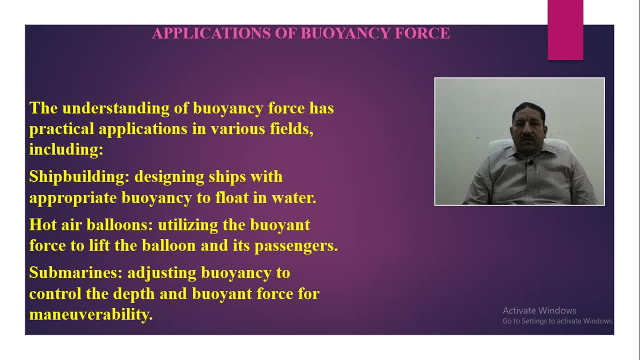 including shipbuilding, designing ships with the appropriate buoyancy to float in the water- I have already talked about this- Ships, etc. are made in a suitable way because their shape and size and volume are taken into account to make them float. All these things are proven. 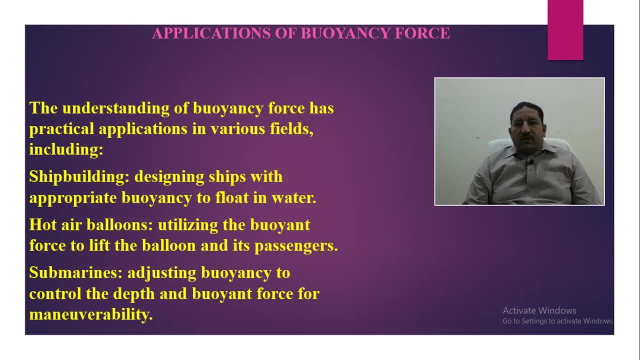 Hot air balloons, utilizing the buoyant force to lift the balloon and express it. This is also an example given Submarines adjusting the buoyancy to control the depth and buoyant force for the. Now these submarines are in the water, So they are also made in such a way that they have a lot of depth. 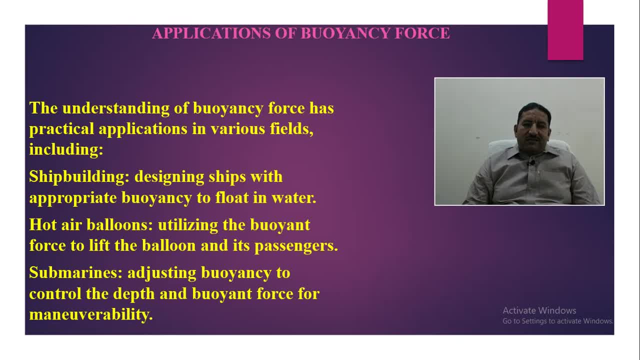 and they are also in the water. So, in this respect, what can you say? they are constructed, they are established, they are made so that the buoyancy force is in control and, in this respect, they are formed to help them float and move.